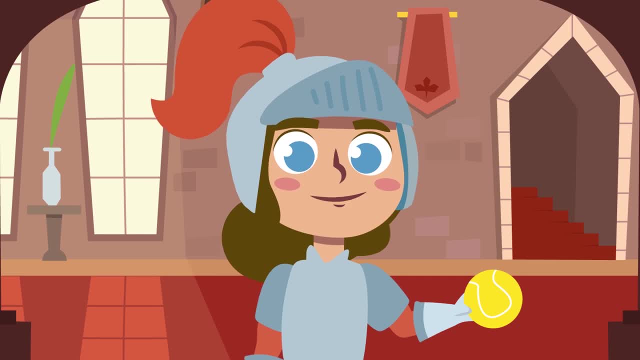 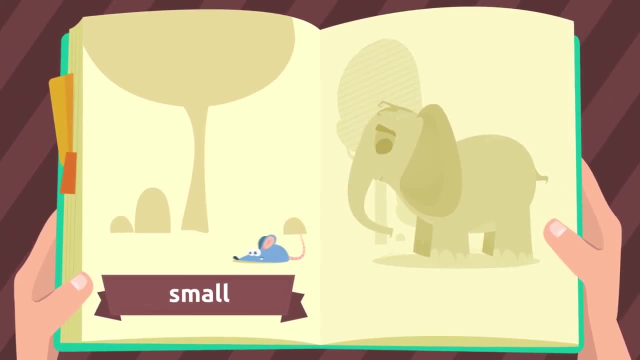 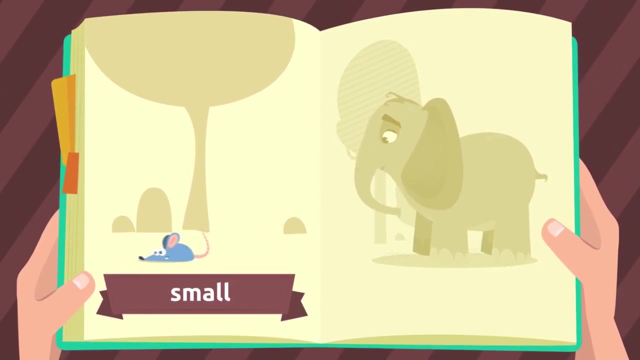 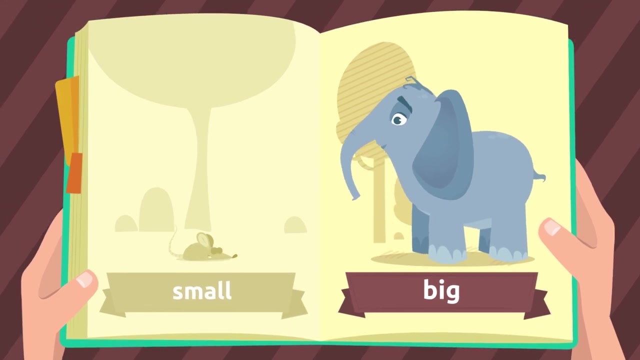 different animals. Come on, let's begin. This mouse is small, Small, Repeat after me, Small, But this elephant is big, Big, Big- Repeat after me: Big, Small, Small, Big, Big, Small, Big. 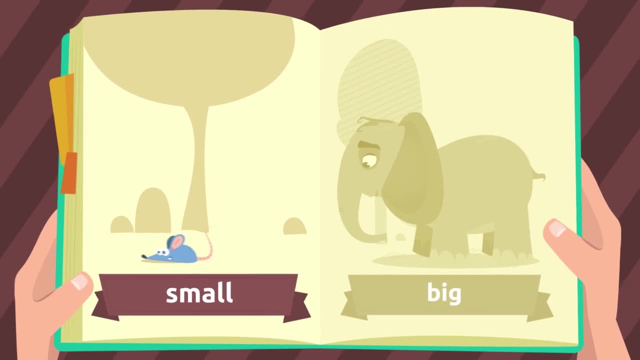 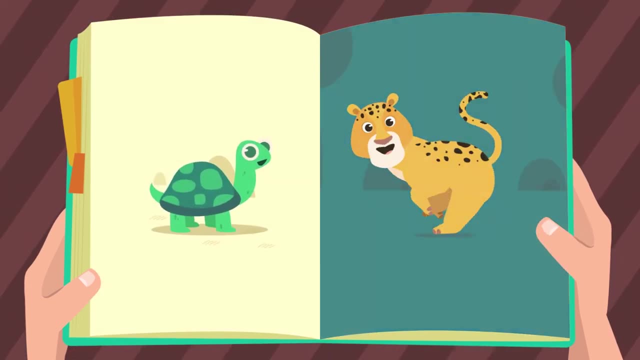 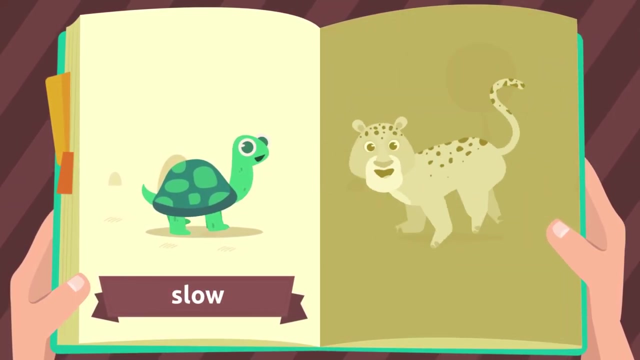 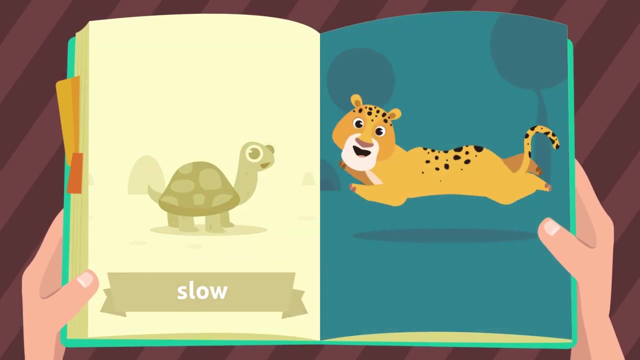 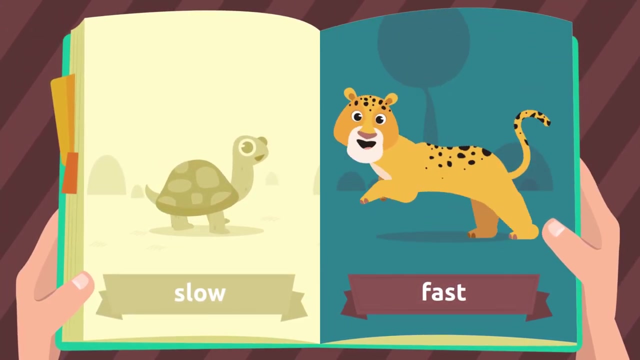 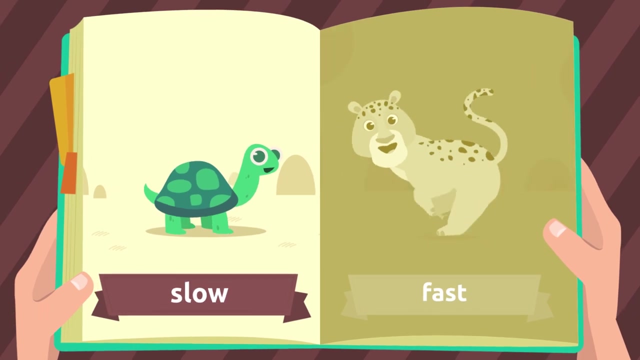 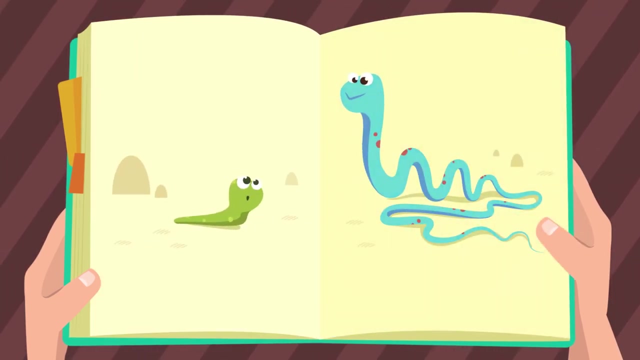 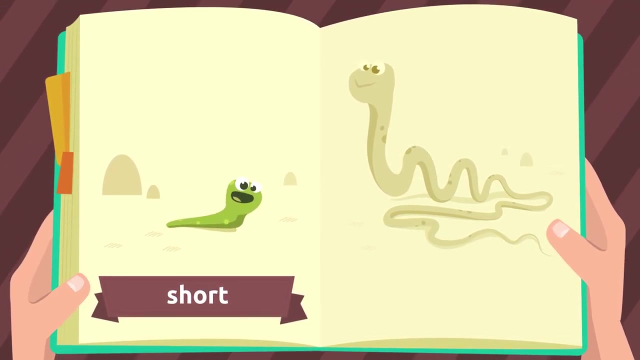 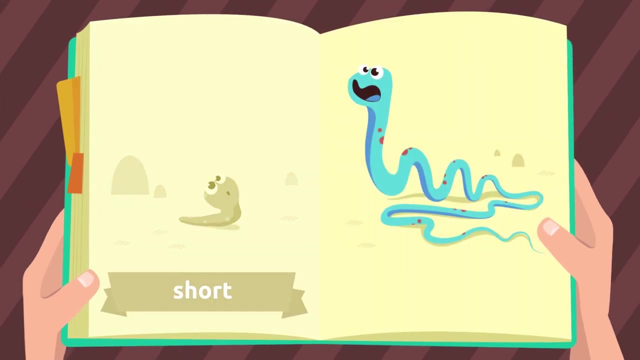 Small, Small, Big, Small, Small, Big, Small, Small. this turtle is slow, slow, repeat after me slow. and this leopard is fast, fast, repeat after me fast, slow, fast. this snake is short, short, repeat after me short, but this snake is long, long. 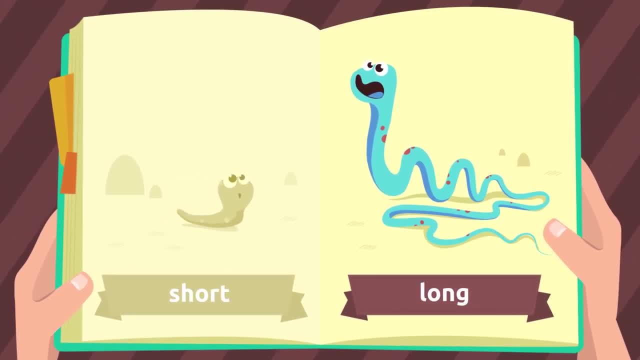 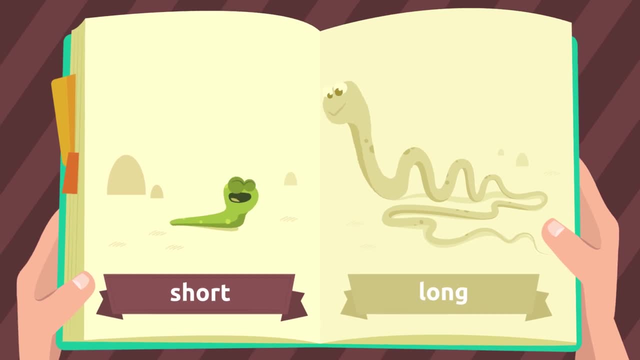 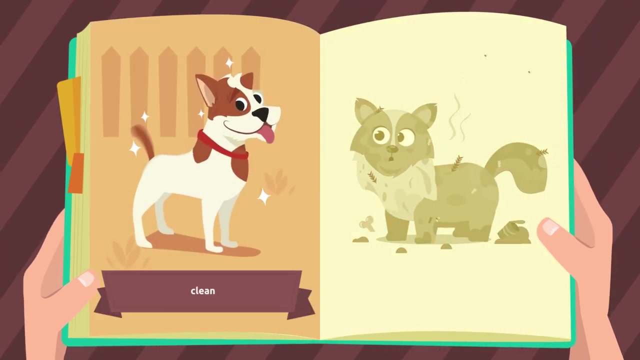 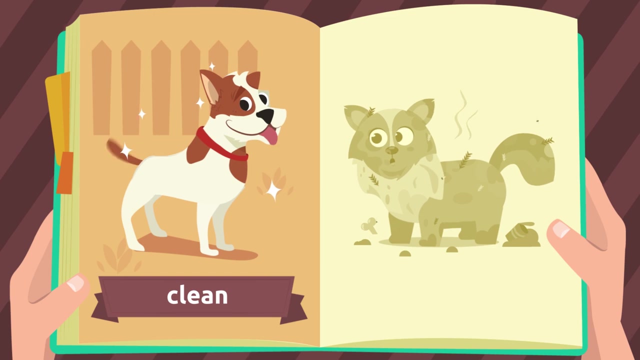 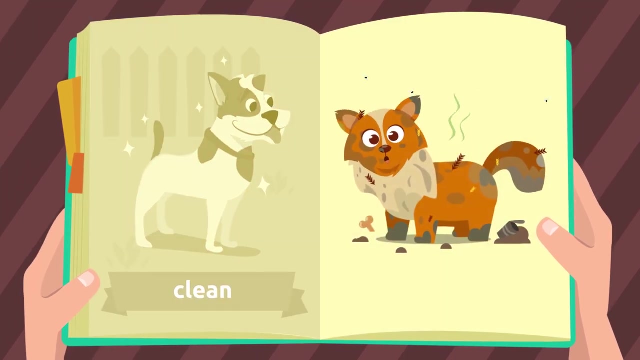 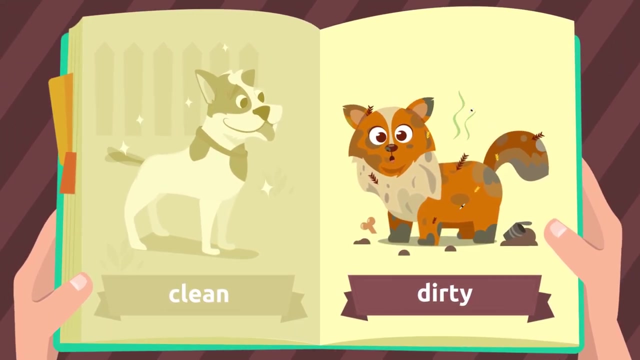 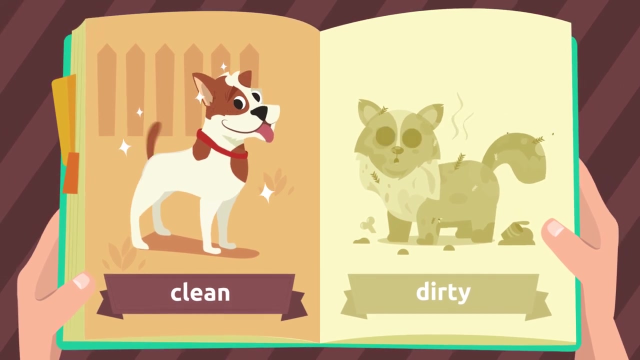 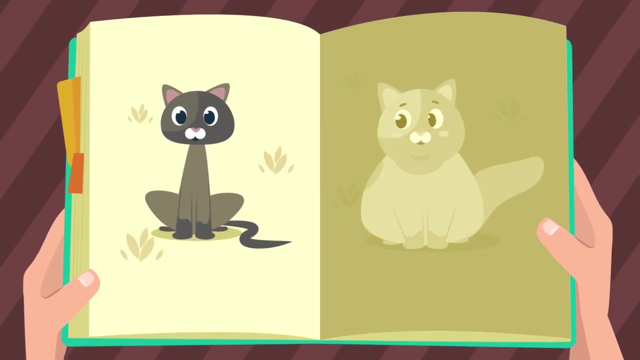 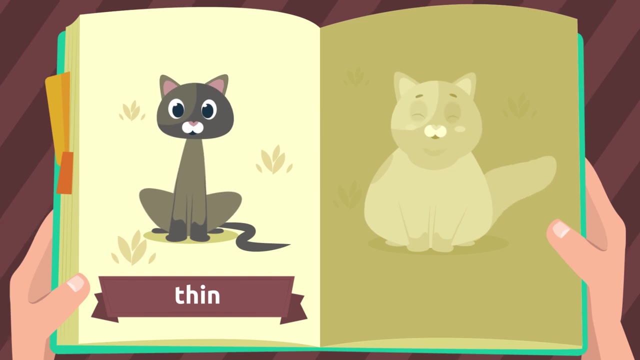 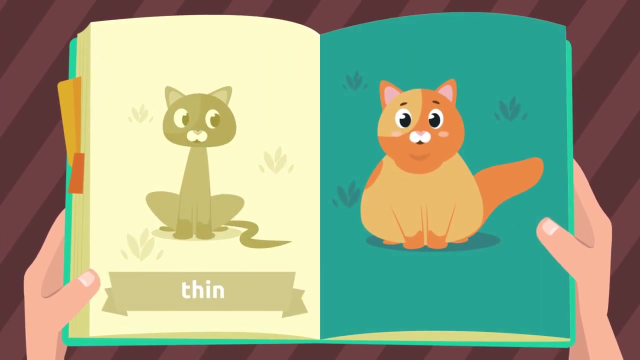 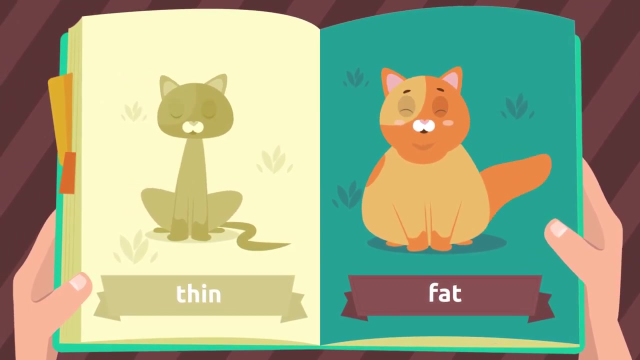 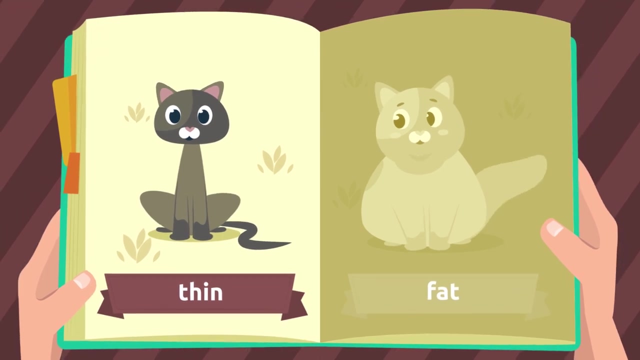 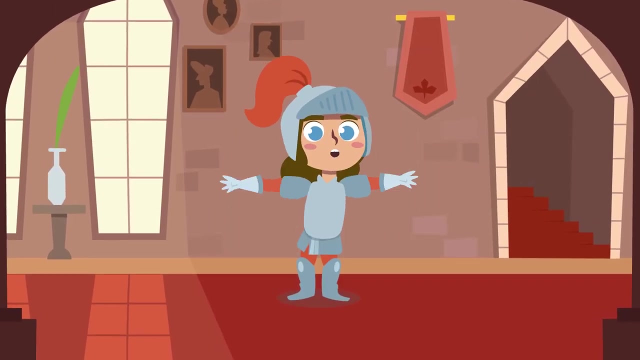 long- repeat after me long, short, long. this dog is clean, clean, repeat after me clean. and this dog is dirty, dirty- repeat after me dirty, clean, dirty. this cat is thin, thin- repeat after me thin. but this cat is fat, fat, repeat after me fat, thin, fat. we've learned a lot of adjectives about these animals. let's review them.